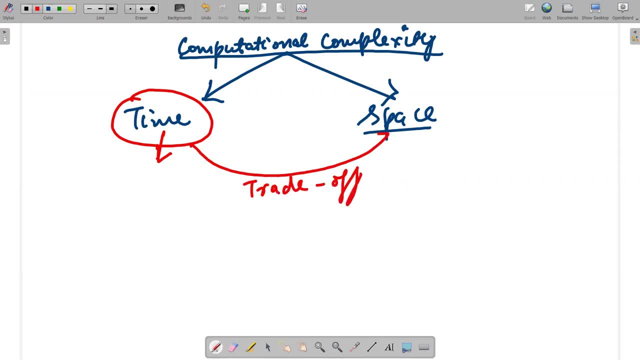 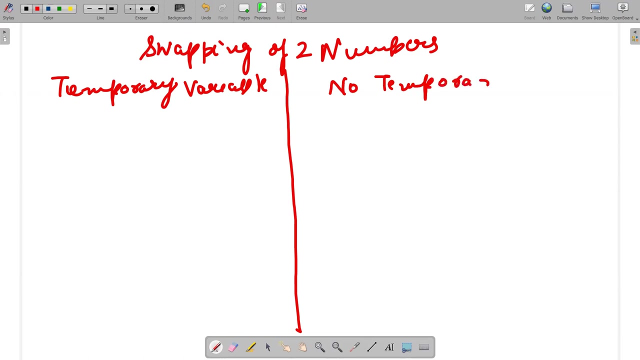 trade off actually happens. So we'll take one example. let's say I'll talk about swapping of two numbers. So if I take this example, so, guys, we all know that this can be done in two ways: If I use a temporary variable And if I don't use temporary variable. So actually it can be done in two ways. 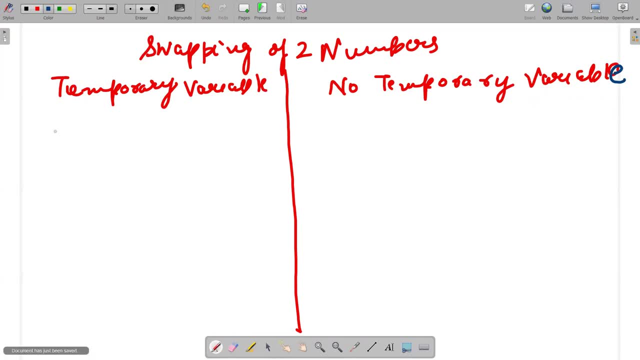 One with the with using temporary variable. if I'm using temporary variable, So let's say the swap syntax would be swap int x, let's say int y, And I'm using temporary variable, int temp, Then I can use the logic of this: temp is equal to x, x is equal to y, y is equal to temp. So this is the logic that I'm using If I'm not using any temporary variable, so I can actually swap two numbers by a particular, particular logic. 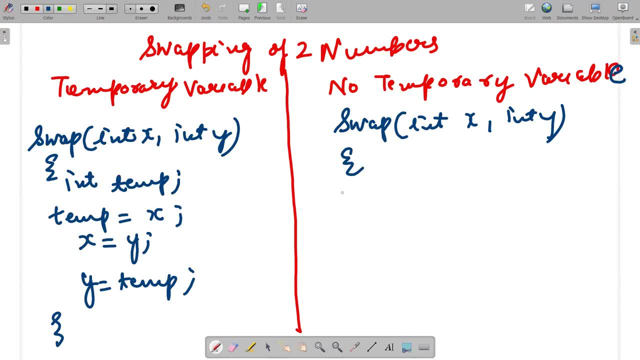 So let's say I'm using temporary variable And if I use temporary variable so I can actually swap two numbers by a particular particular logic. the logic says that i can write: x is equal to x plus y, y is equal to x minus y and x is equal to. 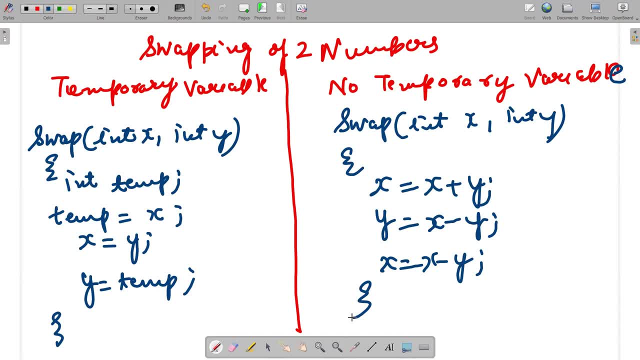 x minus y. again the swapping of two numbers will happen. now why i took this example? because space and time complexity constraints are there in both of them if i take the size of integer as a universal integer variable, as if i just take because size of a width of a variable depends upon compiler. 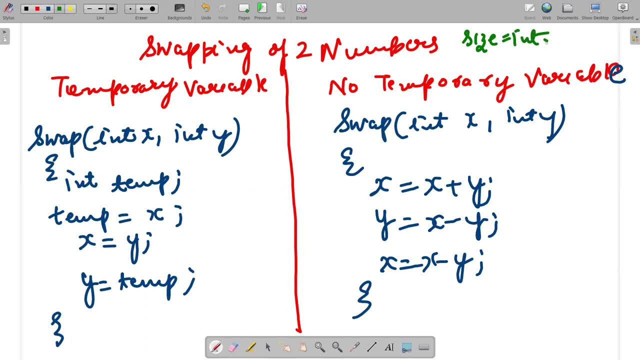 but i'm taking size of integer as two, right? so how i have to basically see if two is the size, two bytes and two bytes are consumed here. so we are using two bytes over here right now. i'm basically doing the operation, so two bytes total. six bytes have been consumed as space. 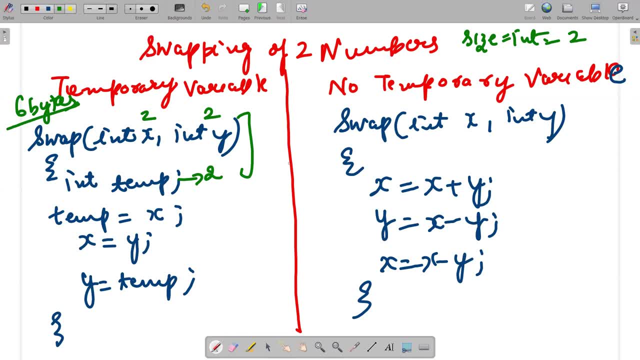 right now i'm just uh from the logic how many steps i'm basically taking from the logic part only, uh, guys, if it is taking one unit of time, if this is taking one unit of time and if this is taking one unit of time, so order of three, uh time. order of three is actually, by default, the order. 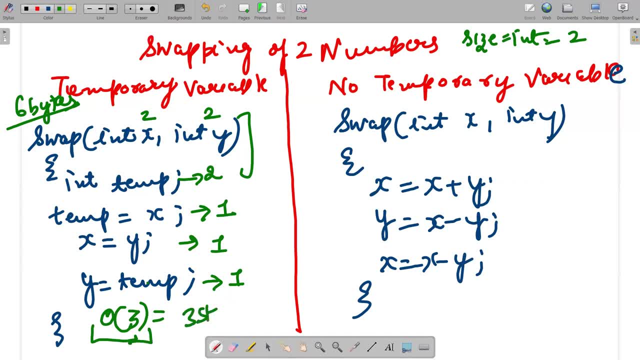 of one. but we are taking how many steps? three steps to solve it. so, as a time complexity, it is taking three steps. now let's come to another part. uh, let's just calculate, uh, the integer size. uh, two bytes over here and two bytes over here. so, technically, as a programmer, it took. 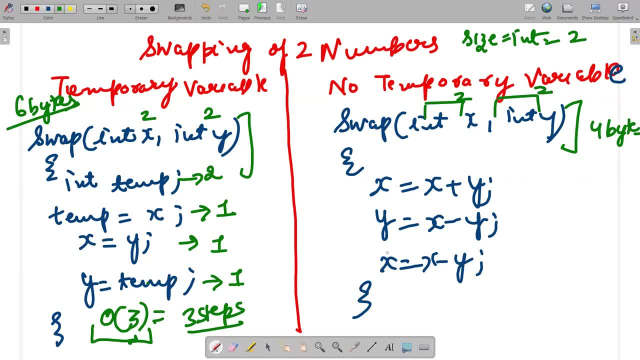 only four bytes. now let's just try to find out how many steps uh of execution is there, guys, as we all know that x is equal to x plus y, so it is something which is: x plus y is assigned to x. so x minus y is assigned to y. x minus y is assigned to x. so firstly, x plus y is computed. 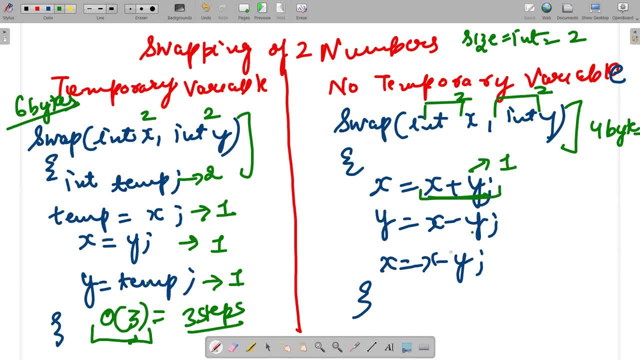 and let's say that computation takes one unit of time and after it is added it is the assignment operation. it means it is assigned to x. so it is taking also one unit of time after calculation of any operation is done. again it is taking one unit of time. after that it is assigned to this. 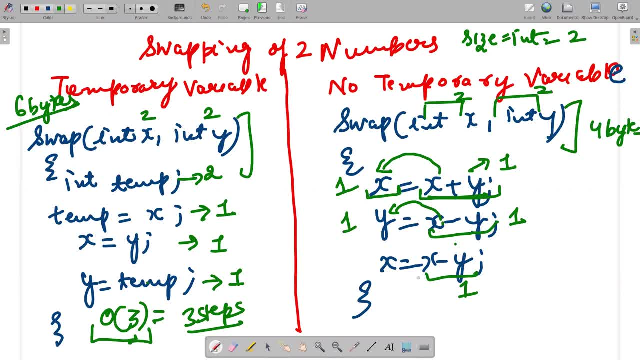 again, that is also taking one unit of time here. one unit of time here, so totally if i basically calculate. so this actually took total six units of time, and over here it means technically we performed six steps, so six units of time. so time complexity of that is order of six and over here time complexity. 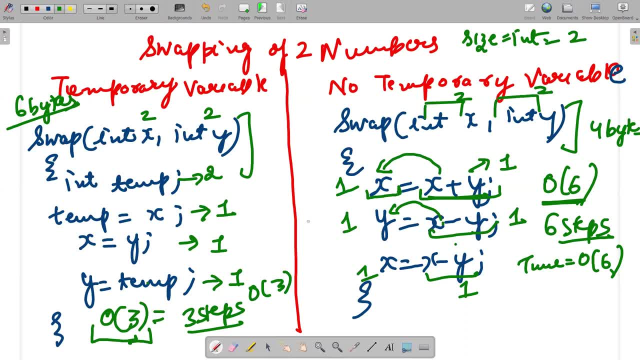 is order of three. i'm not taking the declaration part in consideration. so, guys, it's very, very simple that it is taking six units of time and over here it is taking six units of time as a space. it is covering four bytes. it is taking six bytes of memory, but as a time it